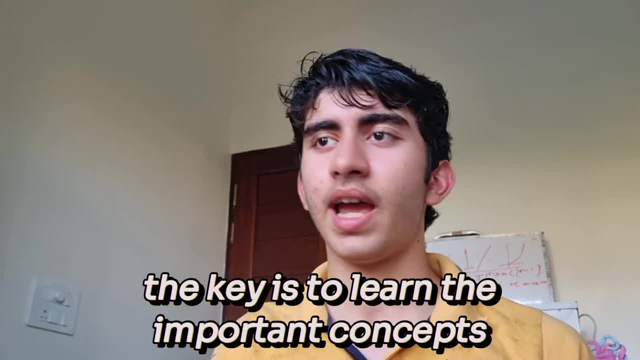 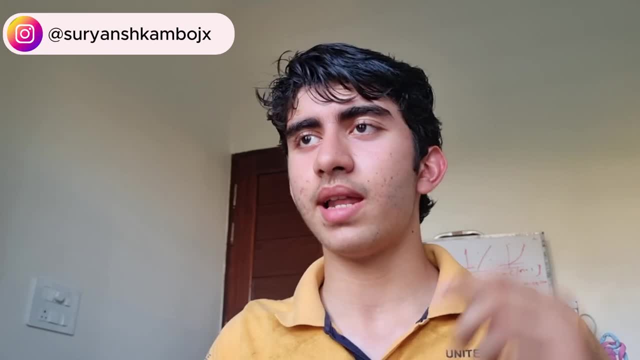 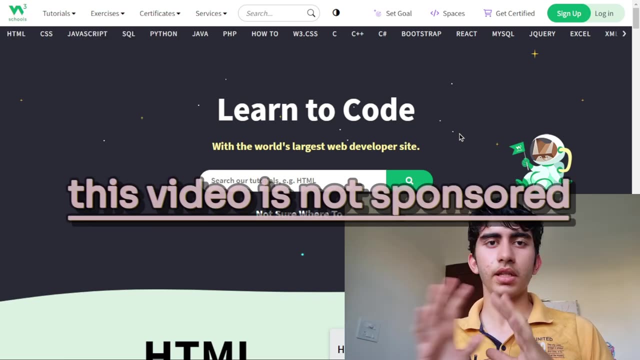 You don't need to just learn everything, and this is the best resource to learn about HTML and CSS. So, without wasting any of the further time, let us see what the website is. So the website is W3schools. This video is not sponsored. Everything is my personal opinion. 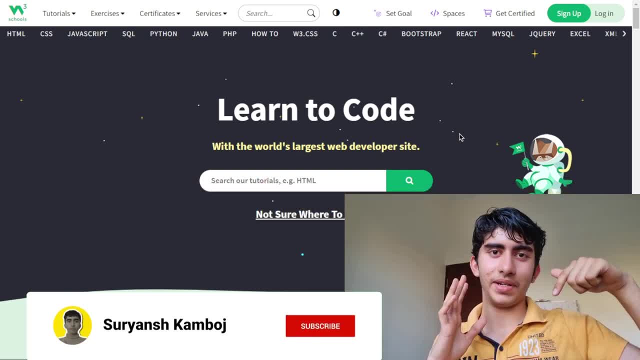 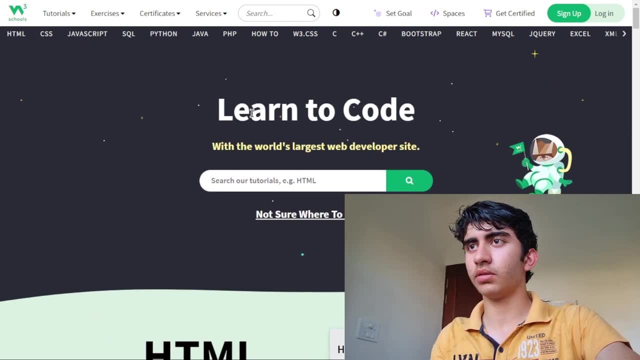 The link is in the description box. You can check that video out, not the video. Check the website out. So, yeah, This is the website That you need to actually learn from, and it's one of the best websites to learn about coding in general, But the thing it's good at it's. 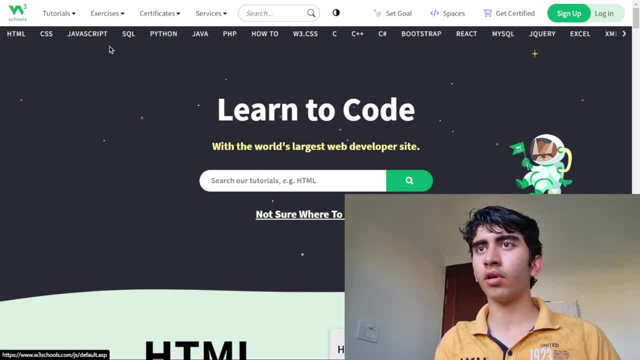 HTML and CSS, Particularly like. I have also tried JavaScript and react from this website, But I don't think it's kind of the best resource to learn from. so I just Love the HTML and CSS of this website and I recommend you to start learning from here itself. 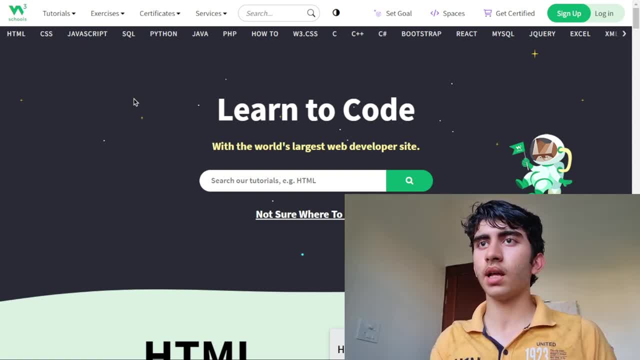 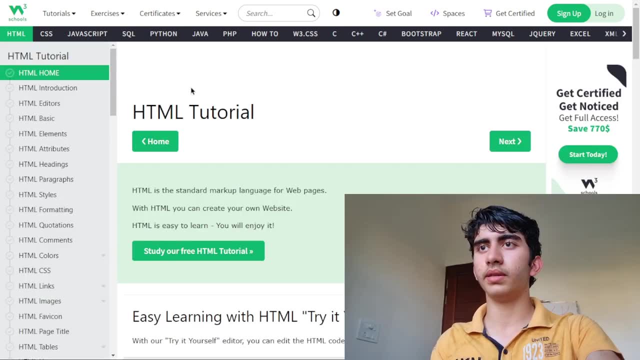 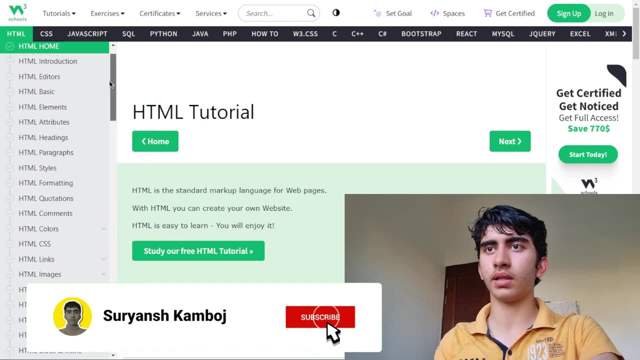 another reason why I chose this Website is like. I'll show you the example. if you click on the HTML tutorial, Then you would be presented with this interface, Which is really clean, first of all, And, as you can see, if you scroll down, you would be presented with this interface like. this is really structured first. 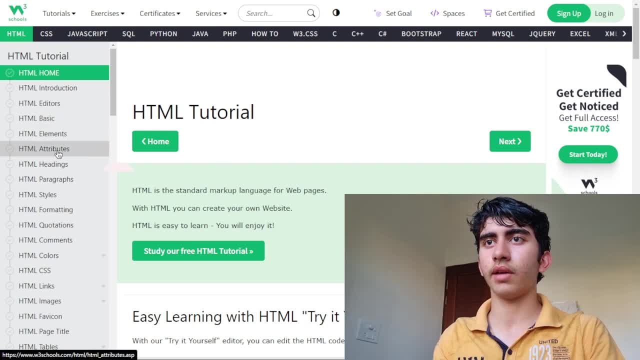 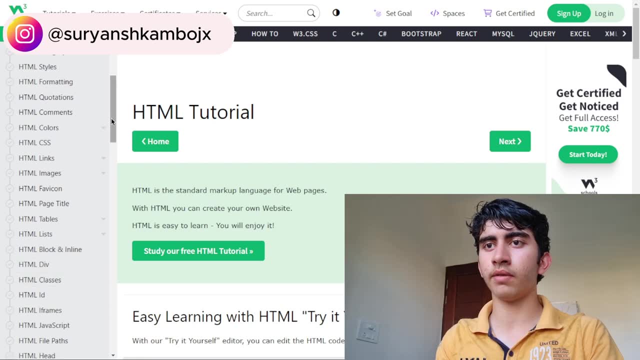 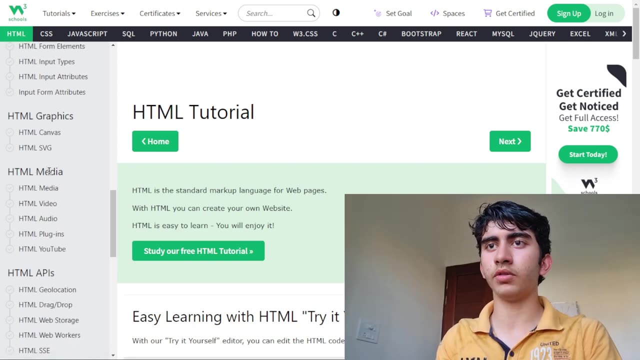 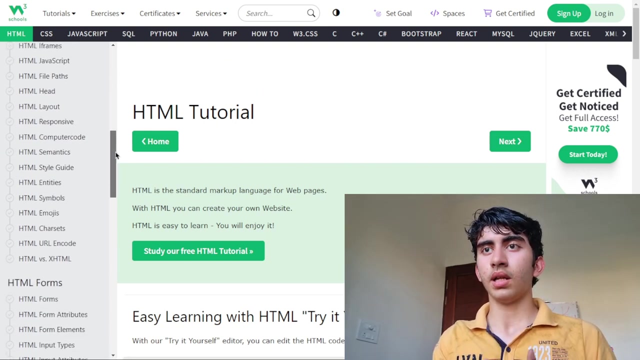 It goes from introduction to editors, like from from really basics, to mediocre concepts like block and inline, what are diffs, what are classes, and then it goes back to advanced concepts like How to use media and HTML, how to use API is even and think advanced concepts like How to use JavaScript. 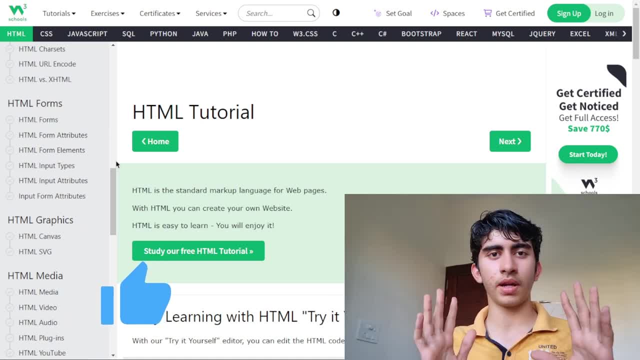 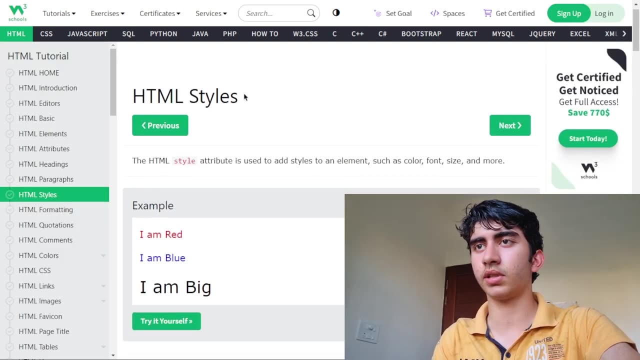 What is XHTML? A lot of advanced concepts for so it goes from really beginner level to advanced level it and it's really structured. another thing I like about this is, if you go on to any of the- let us say- styles for this, for the sake of examples, like you are first of all presented with theory. yeah, so 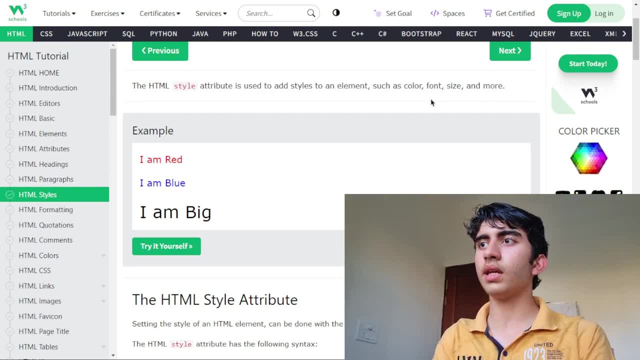 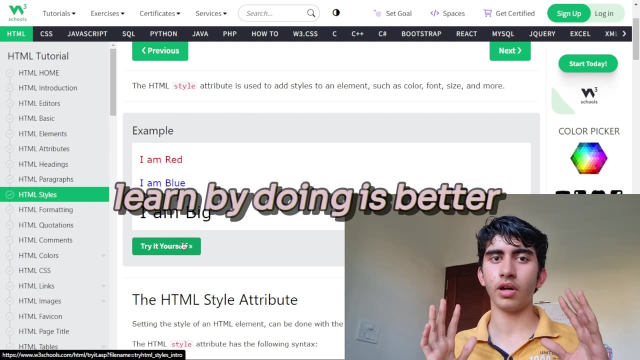 this is, as you can see right here, this is the theory section, and immediately after that there is this example. why is this significant? even you might be asking. this is really important if you are learning by doing, and learning by doing is the best way of learning html, css, because it's. 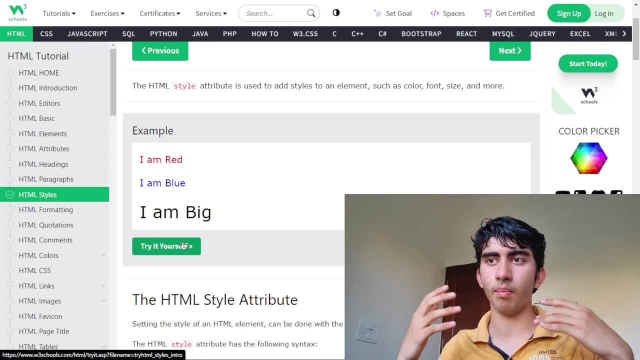 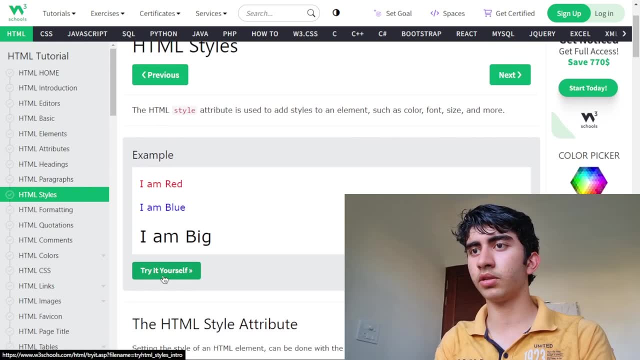 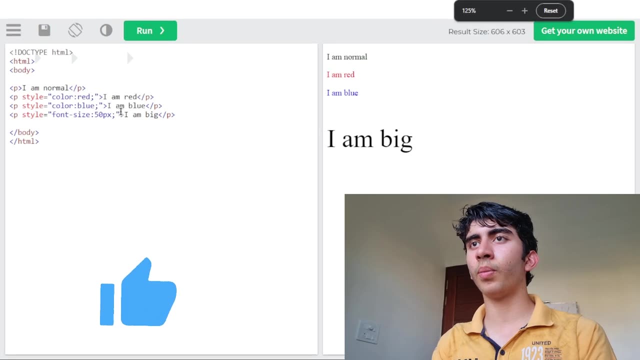 a lot like concepts, memorization, rather than main logic like mathematics. so you are presented with theory and immediately after that you're presented with an example. so you can click on this try it yourself button and you could see the magic happen, like it would open a entire terminal, kind of thing. 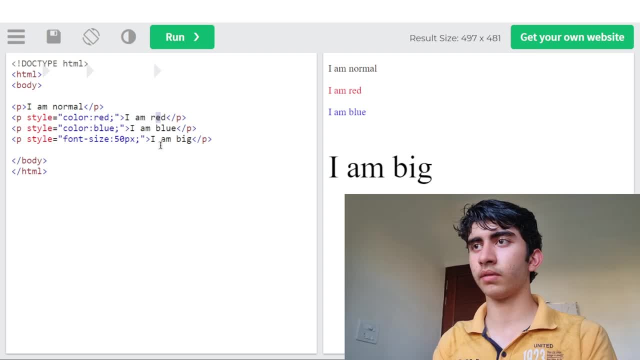 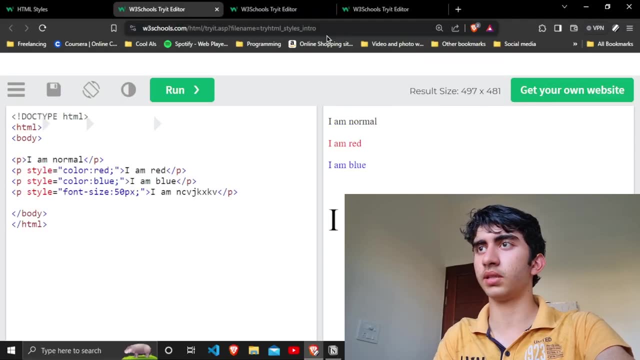 for you for html css, like you can toggle things like from here: i am there, i'll just write something and you can click on this button that would make the changes appear home from this itself. that is why i like this website in general. it gives you a really 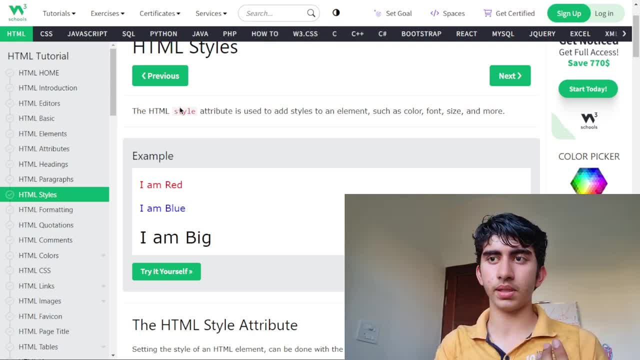 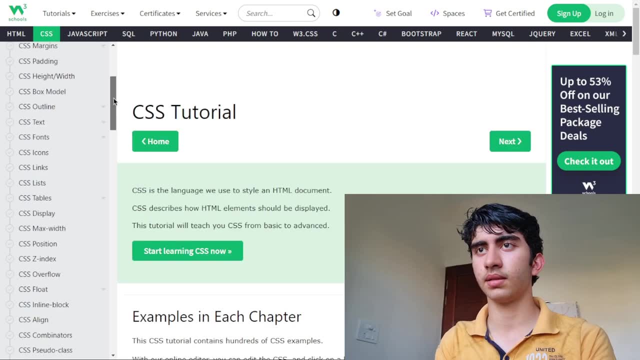 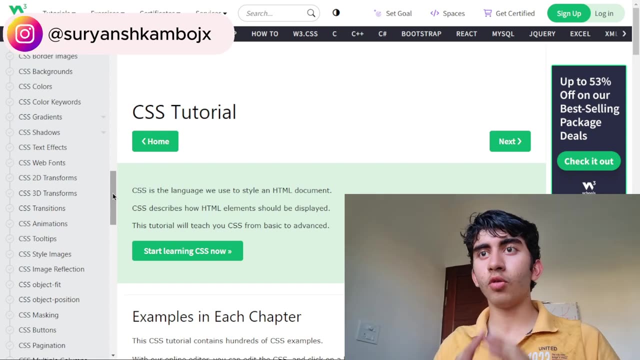 structured way of learning and it provides you with examples and all of the theory in a really structured way. the css section, which i'll be talking about now, is this also very detailed, everything you need to know. also, one thing i have been sharing is: don't go like anywhere else from. 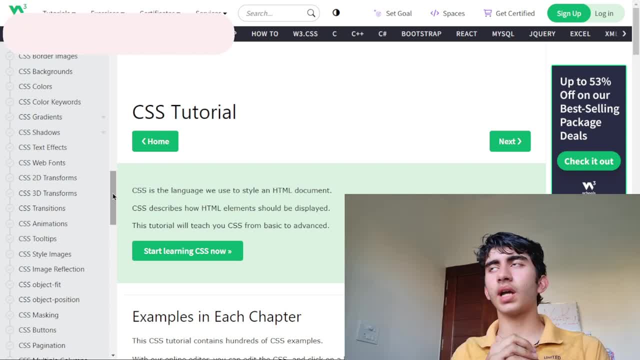 css. after watching this video, like, some people just are so like indulged in html css, they forget about the thing they wanted to achieve. like, if you want to learn about front-end, there are a lot of things like javascript, react, express, there are a lot of things to be mastered. and if you need to know, uh, everything about it, you don't. 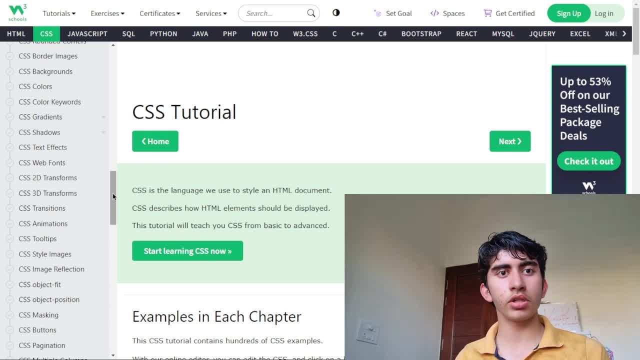 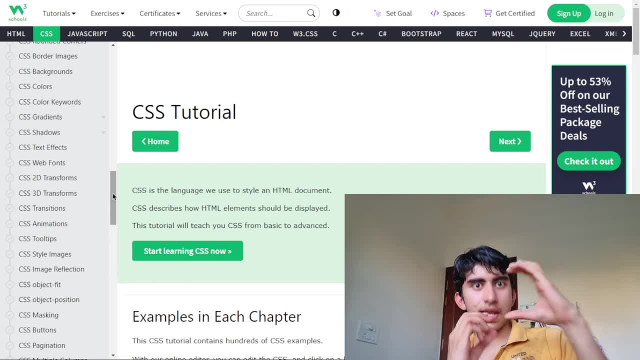 the program. so there are like literal, this thick books on css. i don't know. like, if you learn from this thick books, then when you will be learning about javascript, then react. so, yeah, this is why i chose this website, because, yeah, the structured with and it's like 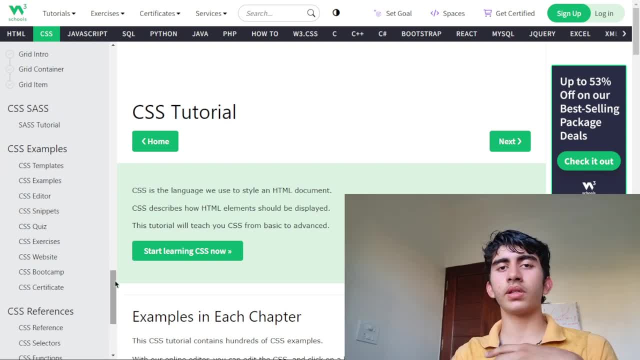 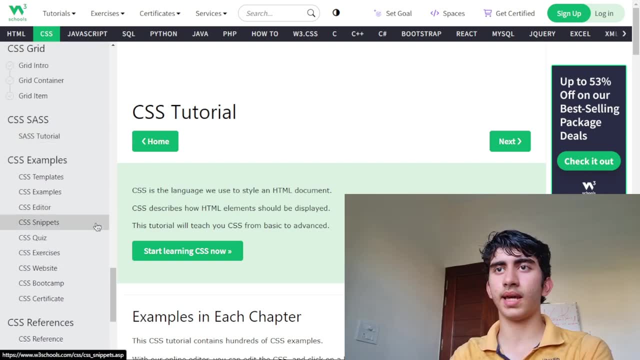 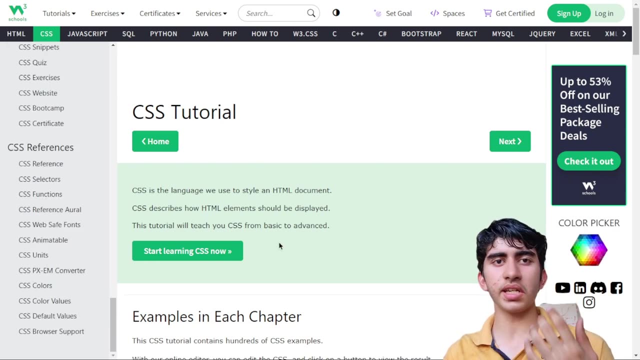 all right, it was now, so you'll be just learning the thing that actually matters you. you can probably skip some sections like this sass tutorial that you can see right here and some concepts that are really not necessary. css is, like, really important to be learned from a good 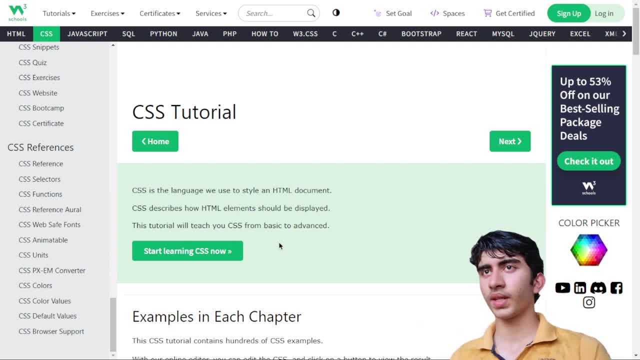 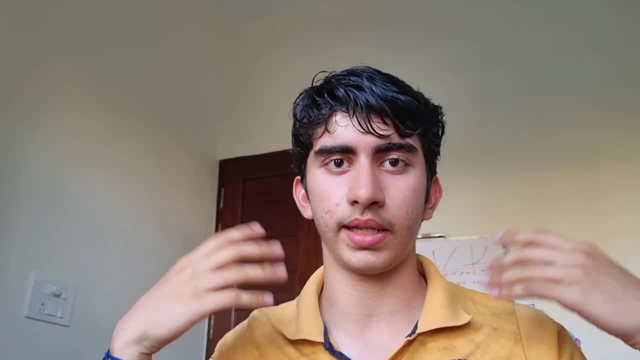 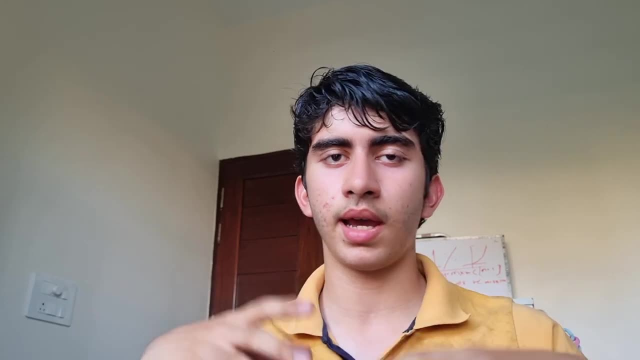 resource, and this is the best resource that i've found. so, yeah, that is all about this website. i hope you like this website. this is not a sponsored video. i'm just sharing that again. so that is all my of my personal opinion. you can have other resources as well, and if you are, if you gain. 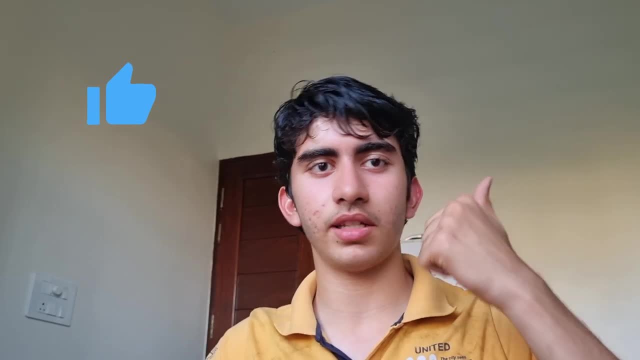 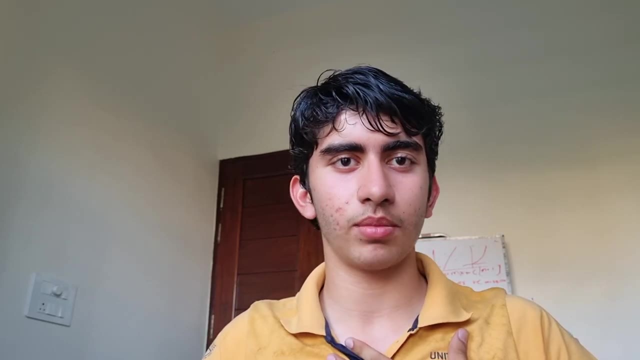 some valuable insights from this video. please make sure to like this video and comment down. i watched till the end to really motivate me to make videos like this one. i am sriyansh kangos. the links to all of this website in the are in the description box after watching the video. 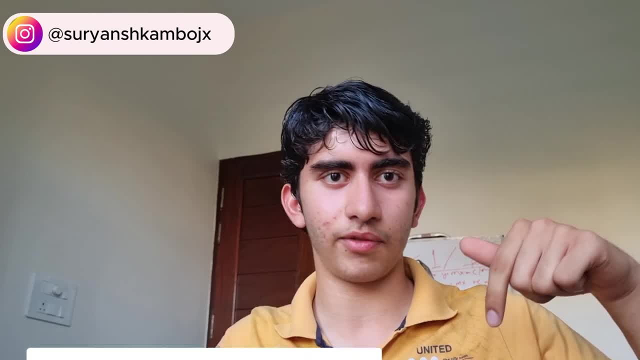 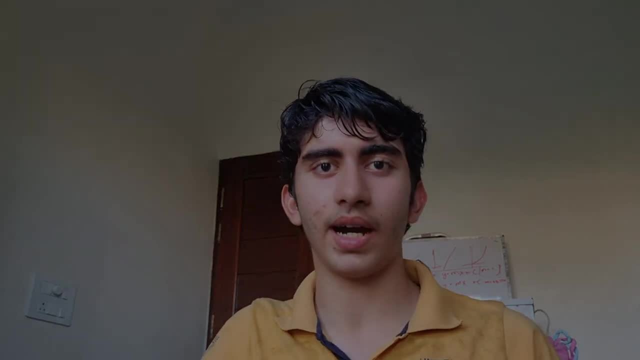 don't scroll uh social media. just start learning your first years about this field. so yeah, all the links are in description. i am sriyansh and thank you for watching this video again, goodbye. 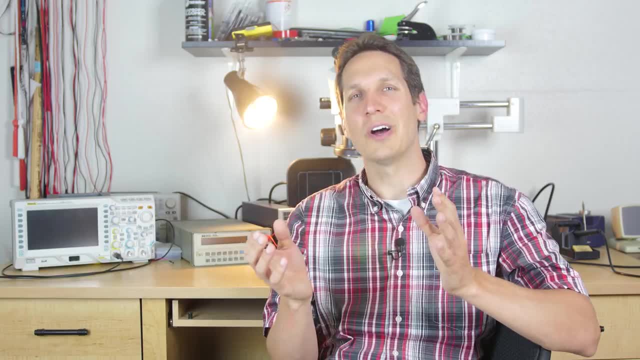 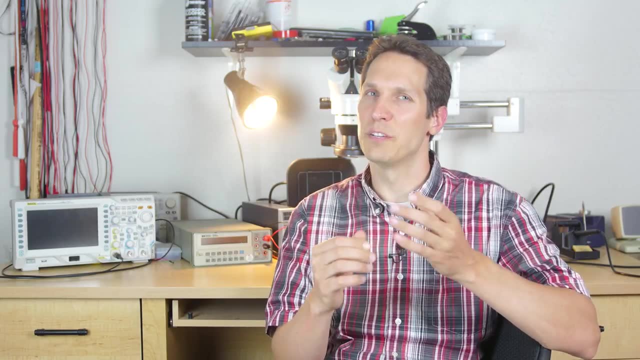 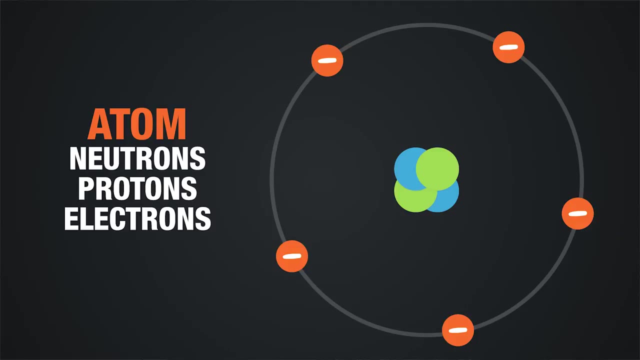 We are going to talk about bandgap and semiconductor current carriers, which will help us understand how current is produced in a semiconductor. If we recall some basic topics in chemistry, we'll remember that all atoms consist of neutrons, protons and electrons, except. 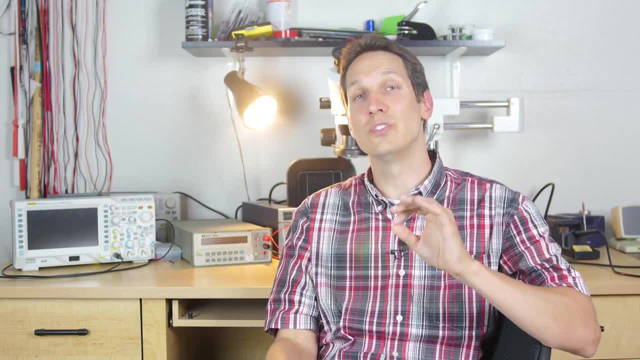 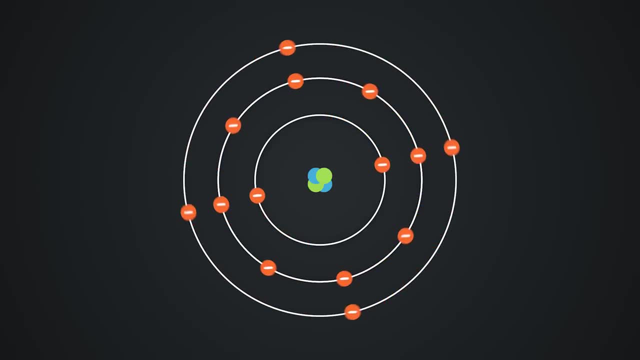 for a normal hydrogen atom, which doesn't have a neutron. Using the Bohr model, we can visualize that an atom has a central nucleus consisting of protons and neutrons that is surrounded by orbiting electrons. The orbits surrounding the nucleus are grouped into 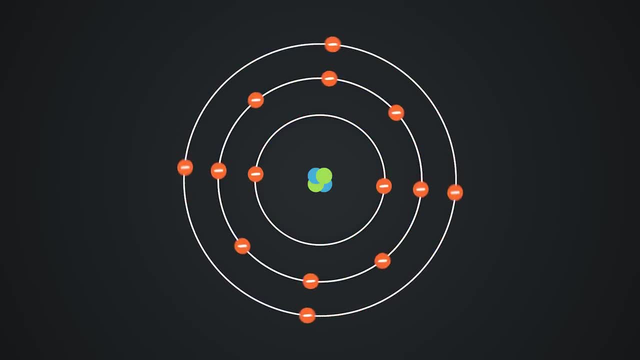 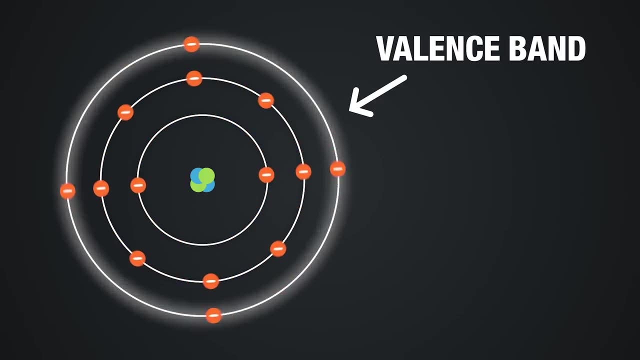 energy levels, known as shells, and the outermost shell is called the valence shell. The valence shell of an atom represents a band of energy levels, which is why it is also called a valence band, and valence electrons are confined to that band. When a valence electron gains enough.